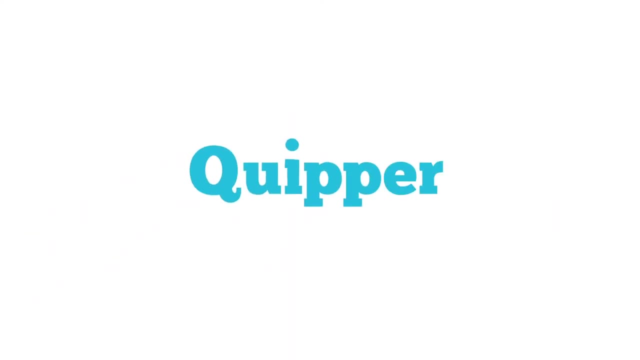 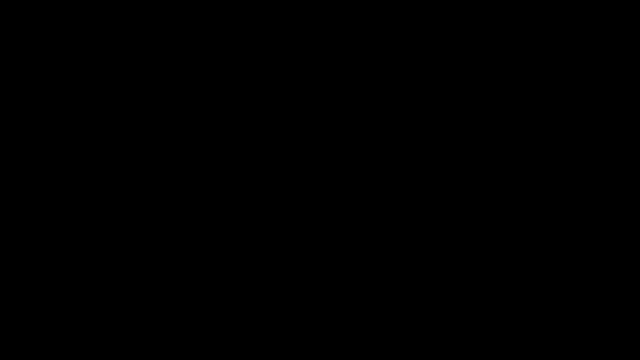 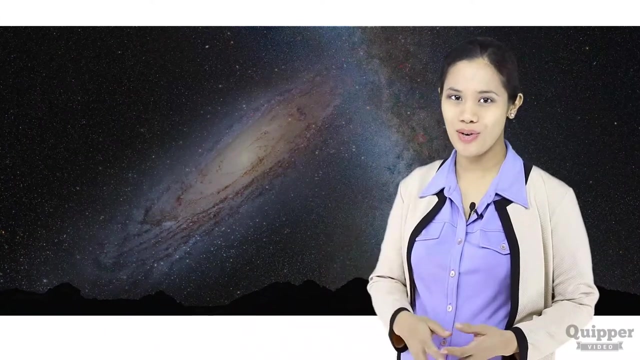 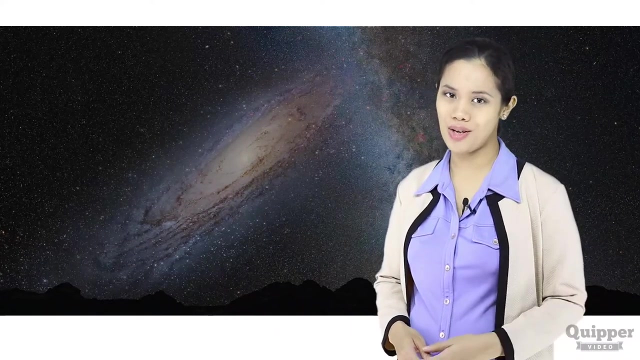 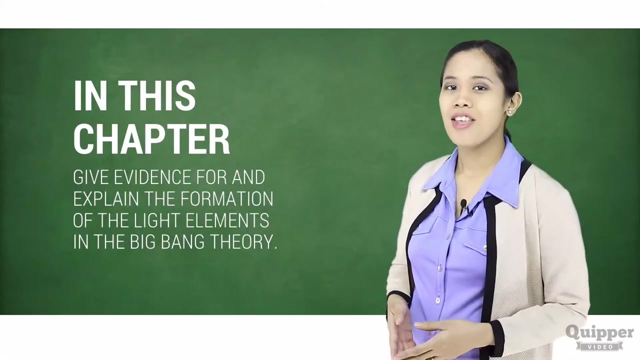 Hello, Welcome to Quipper Video. There are 118 elements that compose our universe, But when the universe began with a big bang, it started out with no elements at all. Where did these elements come from? In this chapter, you will give evidence for and explain the 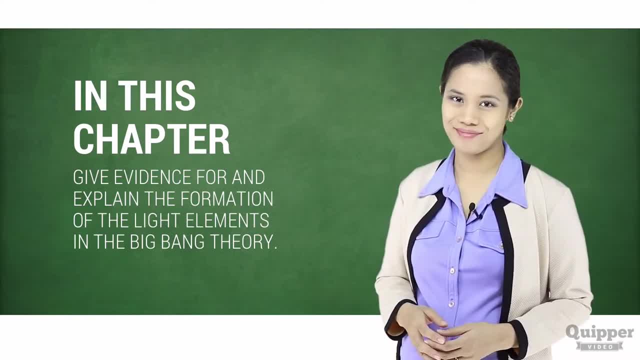 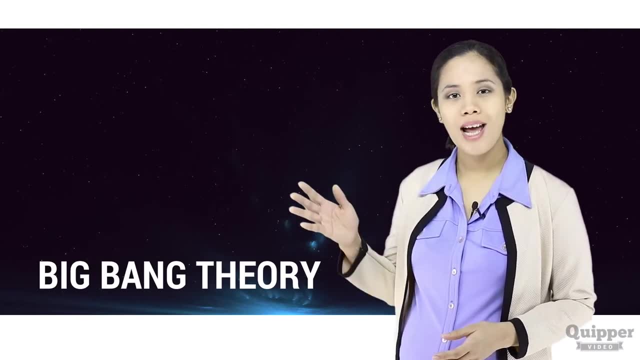 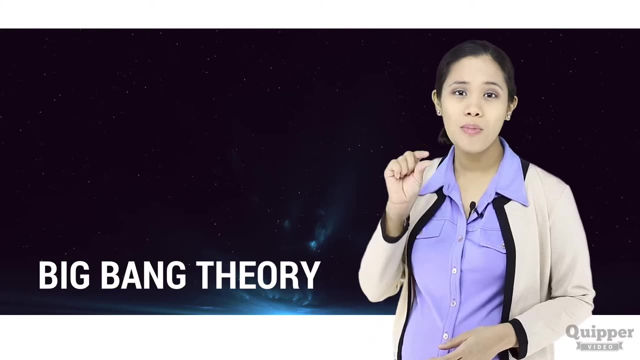 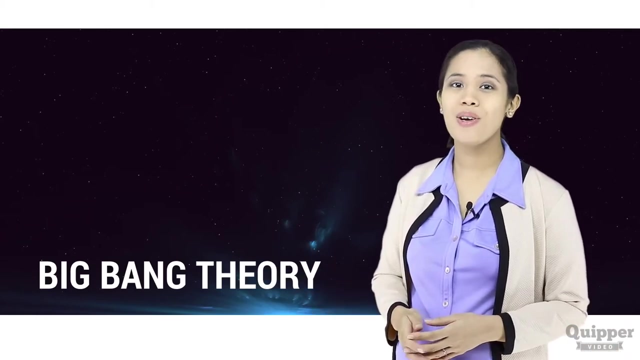 formation of the light elements in the big bang theory. The big bang theory is the leading explanation on how the universe began. At its simplest, it talks about the universe starting with a small singularity, then expanding over the next 13.8 billion years to the cosmos. 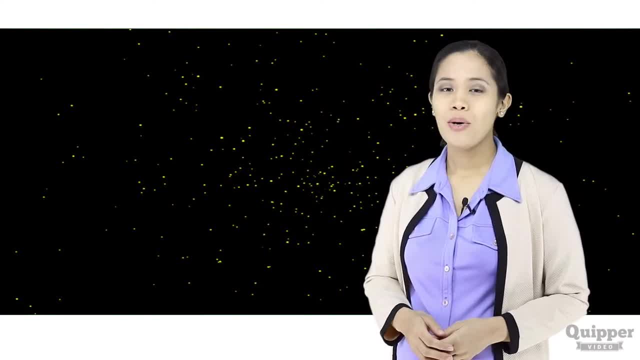 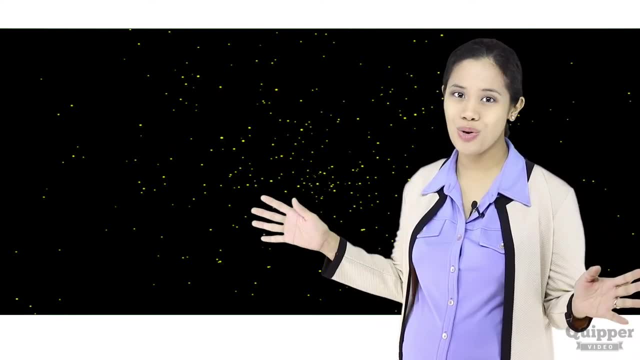 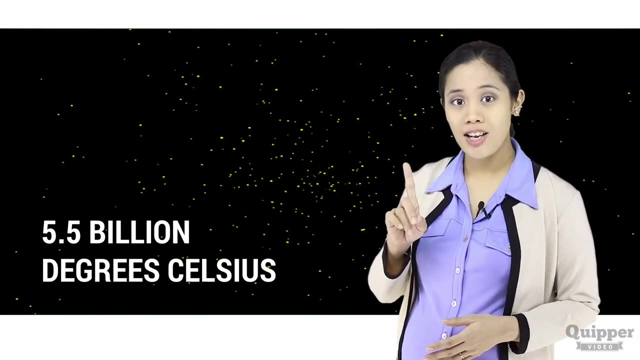 we know today. According to NASA, within the first thousandth of a second following the big bang, all the matter in the universe was in the form of a hot gas of charged particles. Then, in the first second, the surrounding temperature was changed. 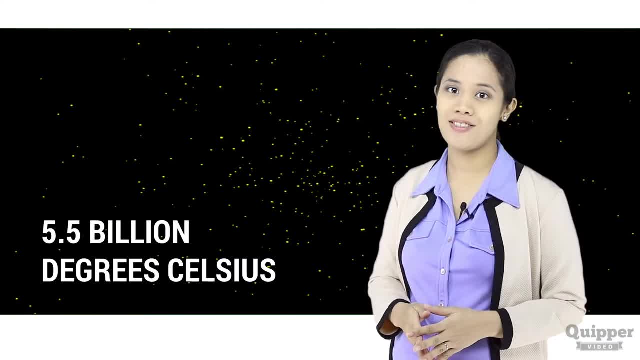 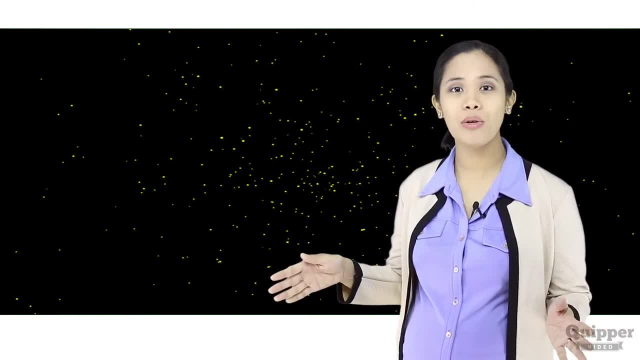 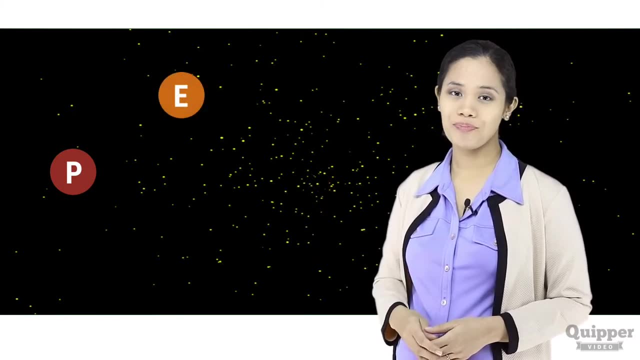 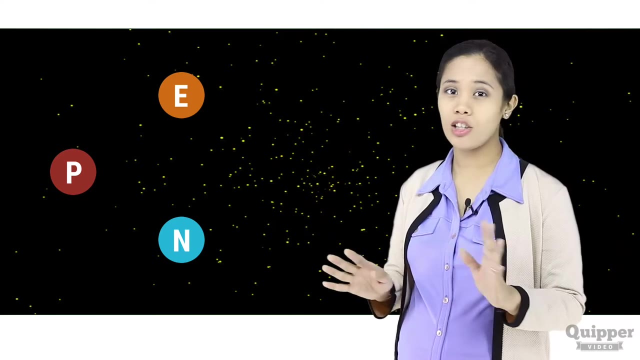 It was about 5.5 billion degrees Celsius. It was too hot and dense. The cosmos contained a huge amount of fundamental particles: Protons, electrons and neutrons. The particles moved about freely and did not come together to make atoms. Only three minutes later, when 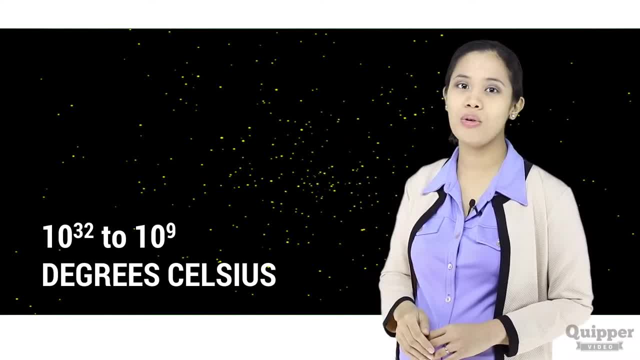 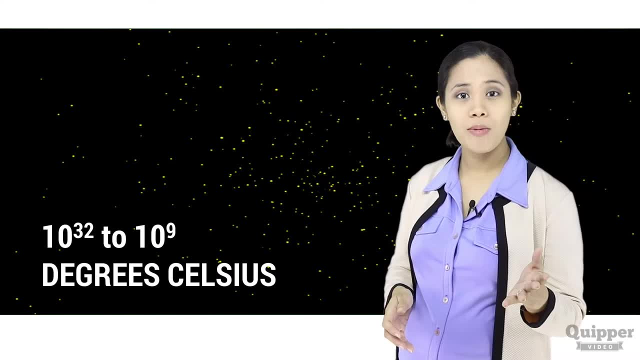 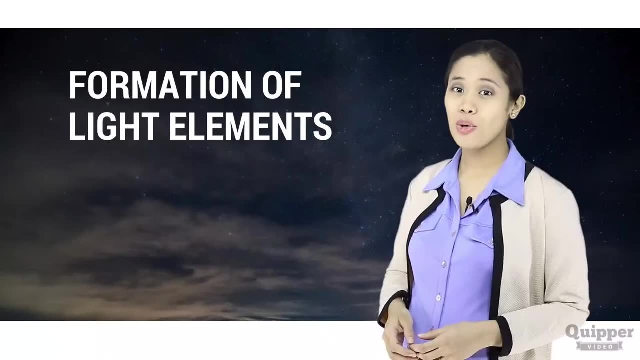 the universe had cooled from 10 raised to 32 to 10 raised to 9 degrees Celsius, did nuclei formation begin. This nuclei formation is known as the big bang nucleosynthesis. Big bang nucleosynthesis, also known as primordial nucleosynthesis, is the process of producing 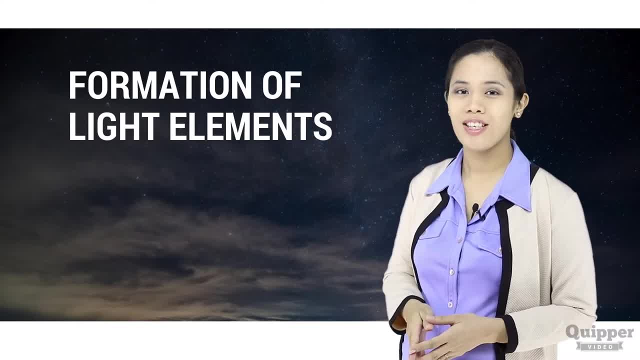 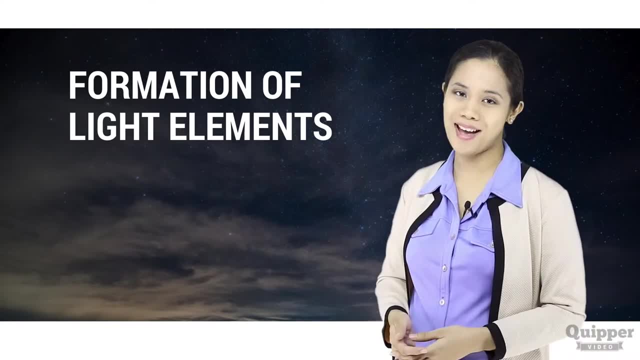 the light elements during the big bang expansion. It is believed to have happened during the 10 seconds between 2.5 and 1.5 billion years ago. The nucleus becomes big bang nucleosynthesis and formed the nuclei of the following elements: 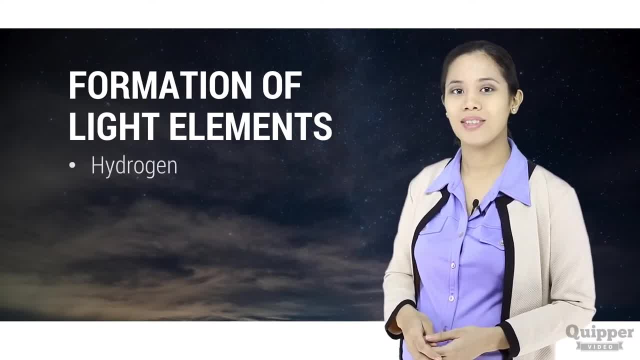 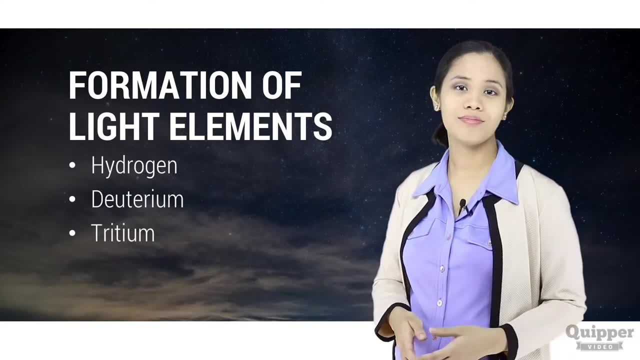 Hydrogen, deuterium, tritium, helium-3,, helium-4,, lithium-7, and beryllium. The material and regions in the nucleus form the nucleus, The heavy elements are the stars, The stars partout. and tears. 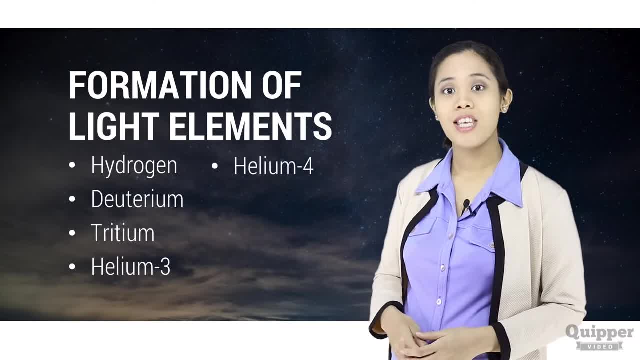 The decimals form the nucleus. The leisures form the stars. The stars form the nucleus. The light elements are the elements. The light elements form the nucleus. The hemoglobin forms the nucleus. The light elements form the nucleus. The imbalances form the nucleus. 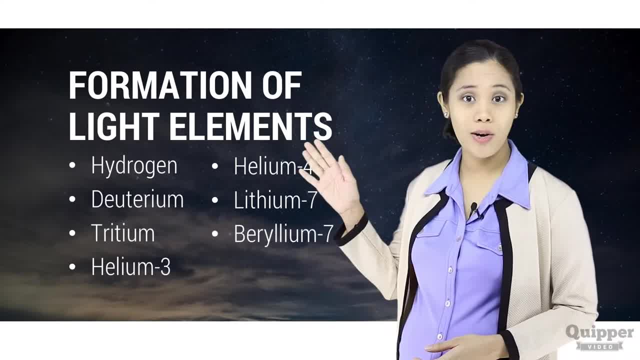 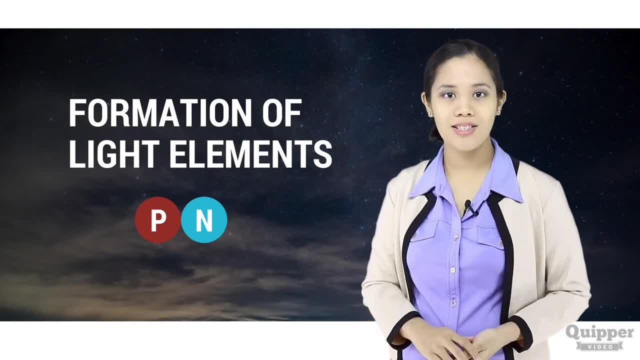 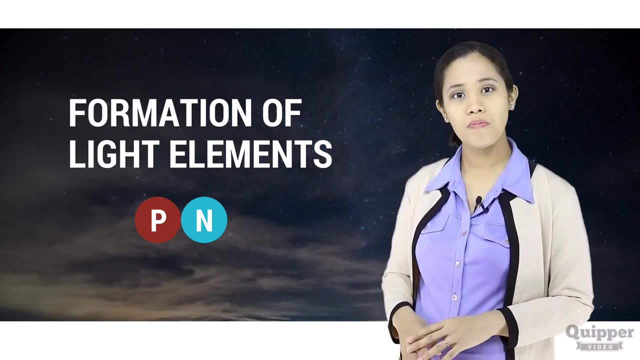 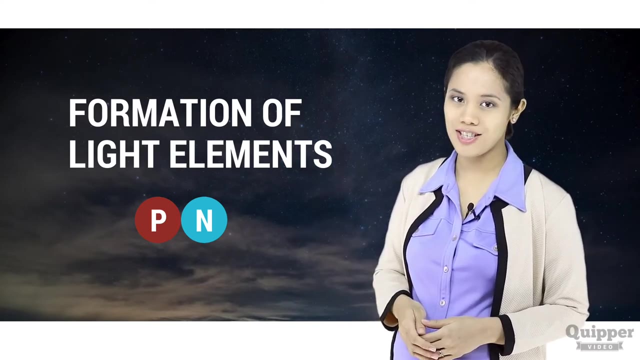 7. remember what nuclei are made up of protons and neutrons. wait, where are the electrons? during the first few minutes after the Big Bang, electrons were still roaming free, so they do not combine to the nuclei yet to form neutral atoms. so let's focus on the nuclei first, as expected, the atomic nuclei of the lightest element, hydrogen, was formed first. what makes up the nucleus of hydrogen? just one proton. so protons were technically the first nuclei. deuterons were the second nuclei to be formed. they are the nuclei of deuterium. they were made when protons and neutrons fused and emitted photons. 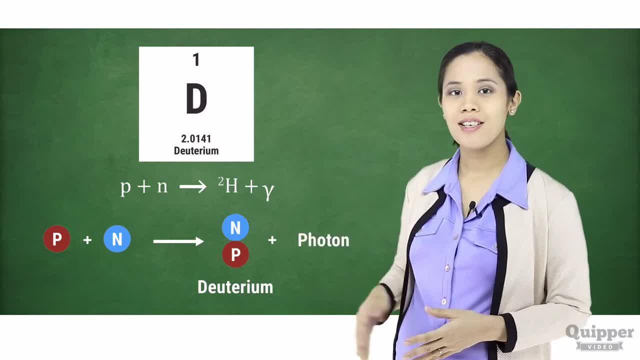 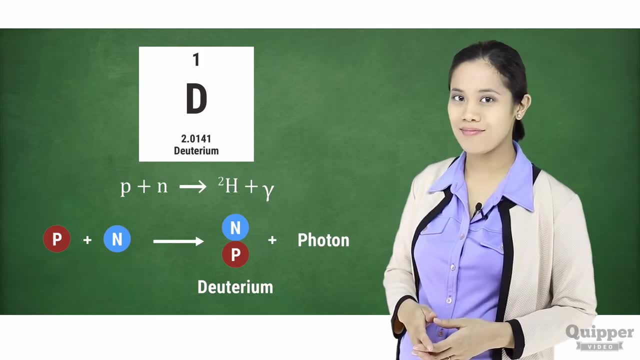 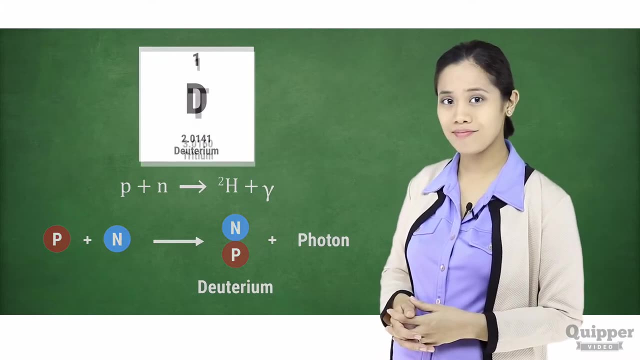 we played around with the number of electrons in the first nucleus. first We can read the nuclear reaction equation as: P or proton plus N or neutron yield, H2 or deuterium nuclei plus gamma rays. Recall that gamma rays are composed of energetic photons. What's next after deuterons? The tritium nucleus. Two deuterium nuclei were fused to create a tritium nucleus with one proton and two neutrons. In this equation you can see that there were no particles lost in the reaction. There were two neutrons and two protons on both the left and right sides of the equation. 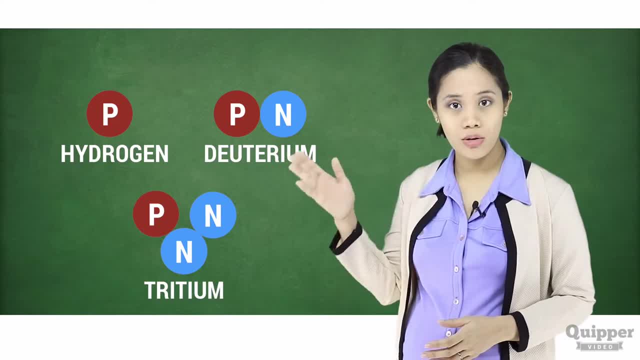 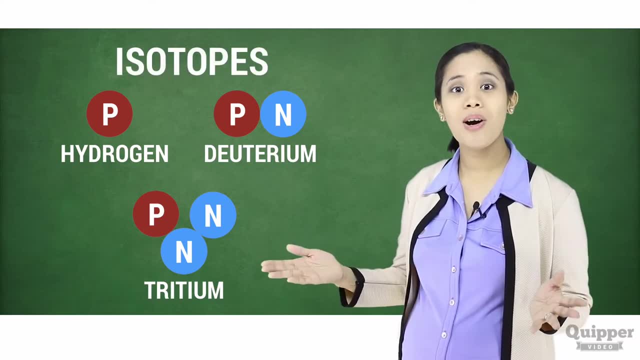 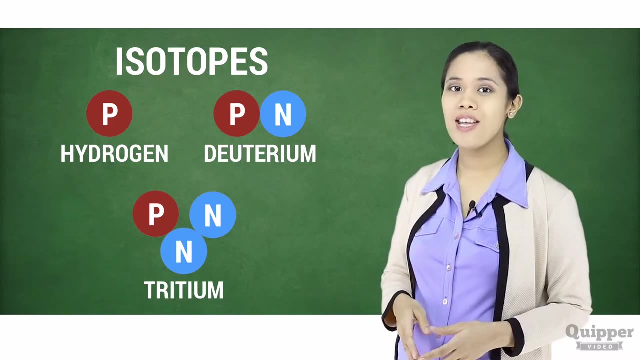 So hydrogen nuclei formed first, followed by deuterium nuclei called deuteron, and then tritium nuclei. Deuterium and tritium are actually isotopes of hydrogen. Remember what isotopes are? Isotopes contain the same number of protons but differ in the number of neutrons. 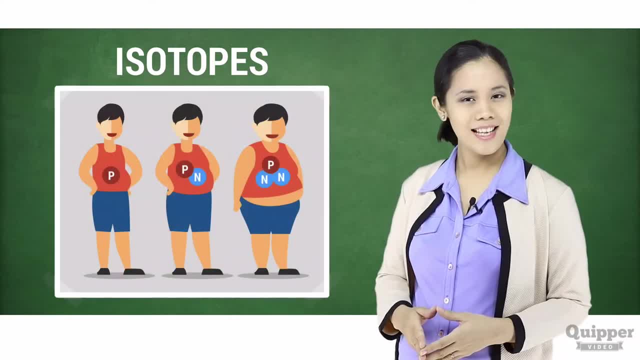 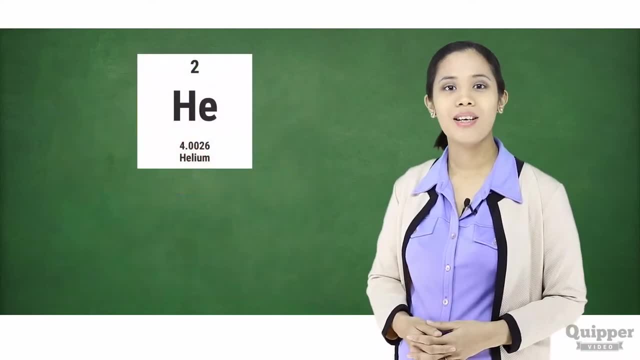 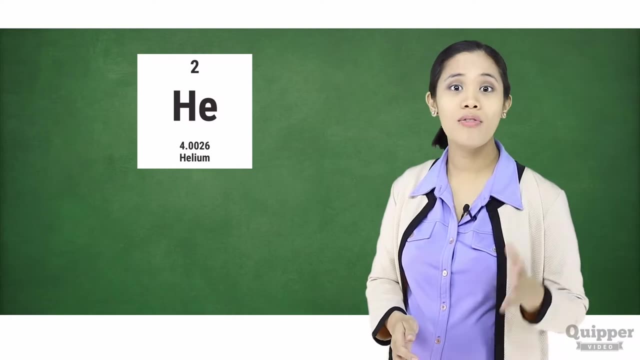 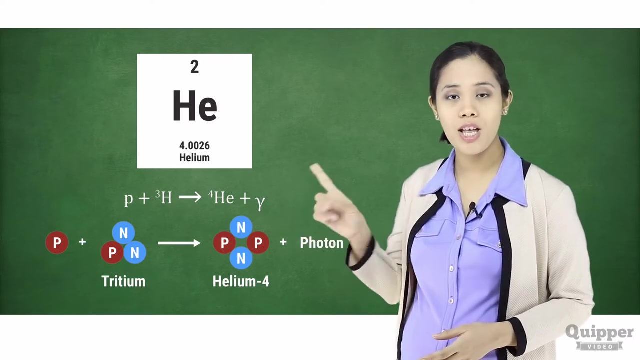 So they have different masses. It's like they have the same identity, but they differ in weights. What happened next after the formation of neutrons, When the tritium nucleus came across a proton, the two particles combined into a helium nucleus with two protons and two neutrons, known as helium-4.. 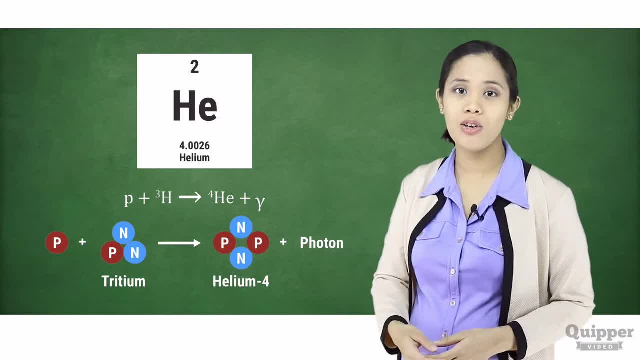 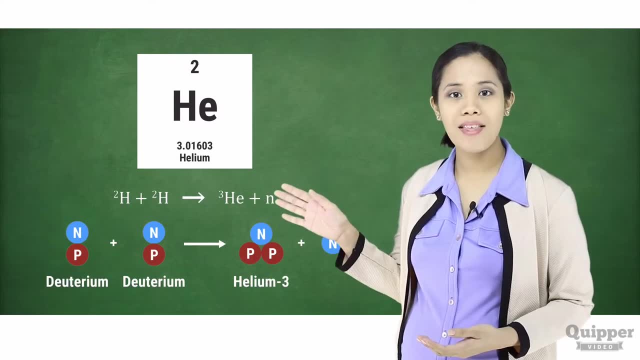 Another path that led to helium was the combination of two deuterium nuclei to produce a helium nucleus. The deuterium nuclei were formed when the tritium nucleus came across a proton. the two particles combined into a helium nucleus known as helium-4. 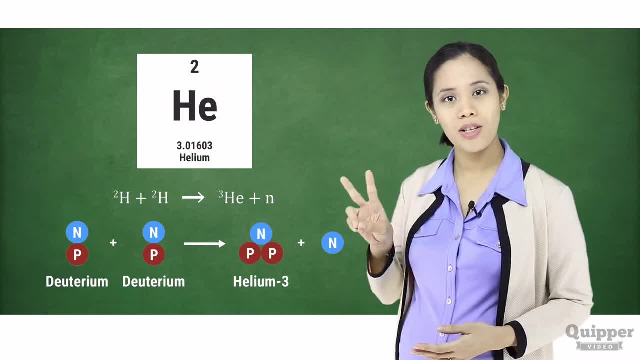 It's the same process as the deuterium nucleus. The new neutron nuclei are the two isotopes of the deuterium nucleus. Here we have a deuterium nucleus and helium-3.. The first, So the deuterium nucleus, has two isotopes, one of which is deuterium and the second. is helium-3. And the deuterium nucleus is made of helium. The two isotopes are created by the isotopes. Helium-3 also has two isotopes. H20 and H41 are also ion isotopes. The isotope is also an isotope. The isotope is a solid. The isotope is a solid And in the system of helium-2, helium-3, there are two isotopes. Helium-3 can be converted to helium-4,, the more stable isotope. 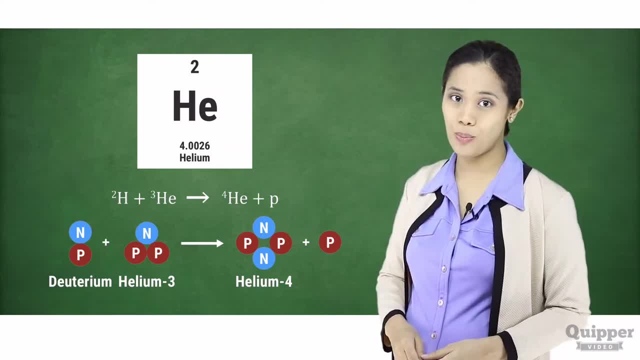 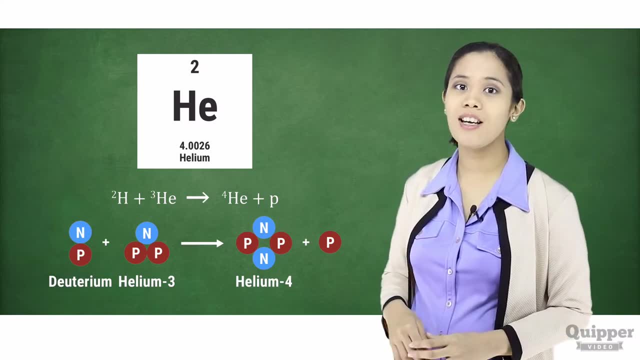 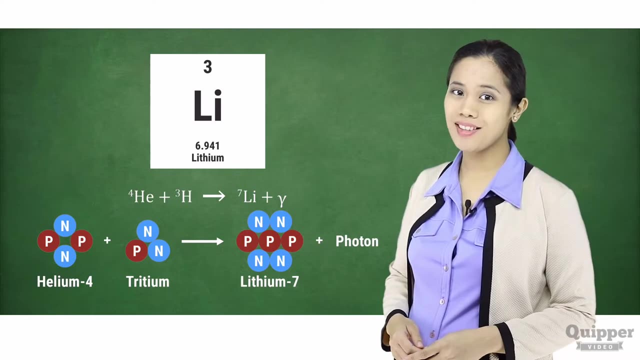 But what happened here? 4, the more stable isotope. When Helium 3 came across a deuterium, they fused to form a Helium 4 and a proton. After the formation of Helium, the nuclei of the next element, Lithium, were formed. 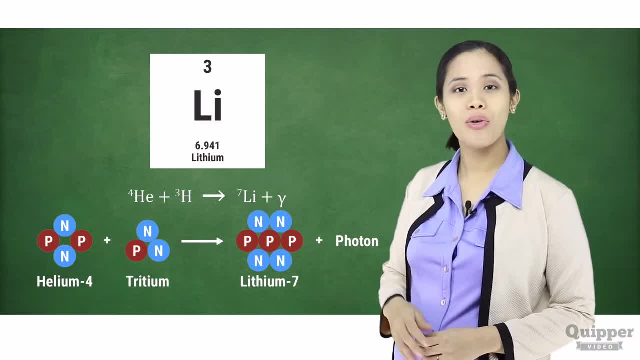 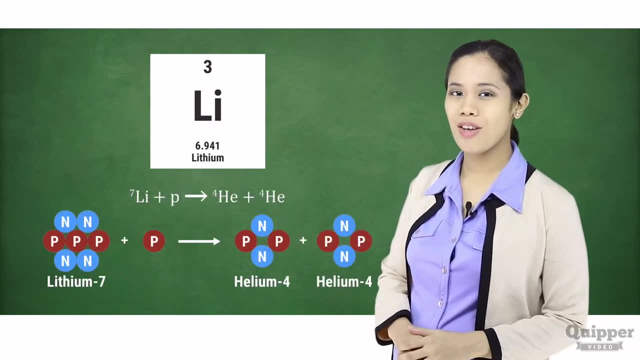 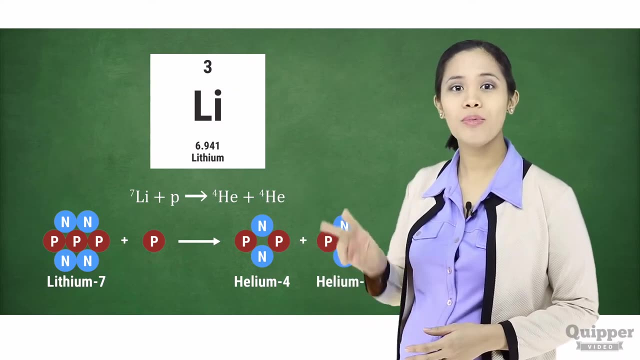 Lithium 7 was produced from the nuclear fusion of Helium 4 and Tritium. It has three protons and four neutrons. Lithium 7 was actually unstable, so right after its formation it decayed spontaneously to form two stable Helium nuclei. Another unstable nucleus that formed was Beryllium 7,, which has three neutrons and four protons. It was produced from the nuclear fusion of Helium 3 and Helium 4.. In the case of the Beryllium 7,, it was produced from the nuclear fusion of Helium 3 and Helium 4.. In the case of the Beryllium 7,. it was produced from the nuclear fusion of Helium 3 and Helium 4.. Being unstable, it decayed spontaneously to Lithium 7 by releasing a proton. The early soup of particles would have been impossible to look at because there was no light shining through it. About 380,000 years after the Big Bang, the universe cooled down and the particles began combining to form neutral atoms. About 380,000 years after the Big Bang, the universe cooled down and the particles began combining to form neutral atoms. Their combinations allowed light to shine. Yes, the first neutral atoms were formed, But these were only the two lightest elements, hydrogen and helium. That's pretty much it. It took a billion years before the next element of the periodic table, the neutral lithium atom, was formed. 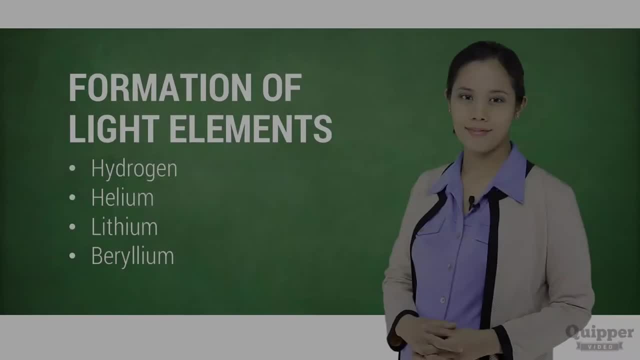 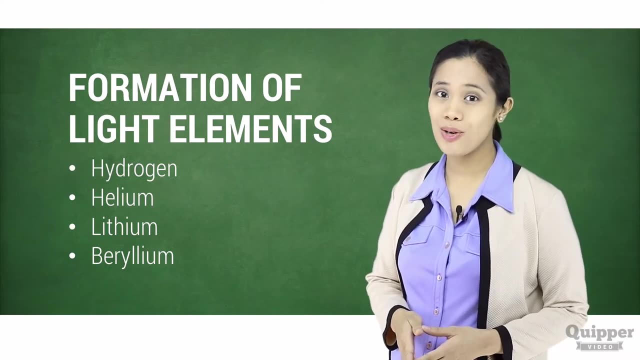 Such a long time for waiting. So hydrogen, healed Helium, lithium and beryllium were formed during the Big Bang- nucleosynthesis, according to astrophysicists. Now the question is, what made them think so? 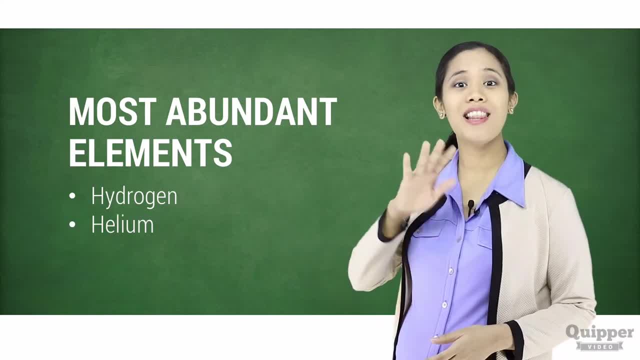 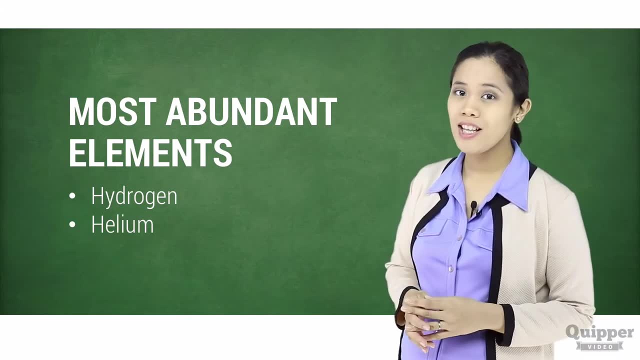 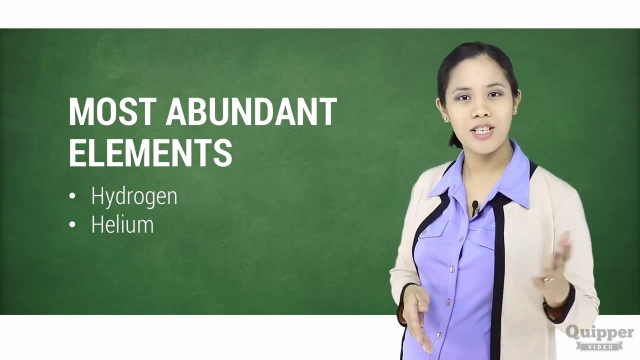 Their answer is the abundance of the light elements. Scientists calculated the abundances of primordial material based on the Big Bang theory. They found out that the total mass of the universe would have been 25% helium, 0.01% deuterium. 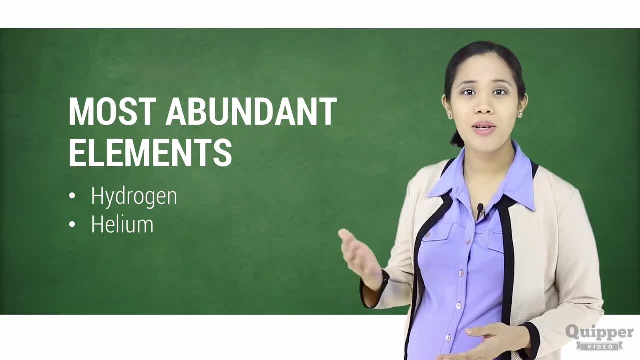 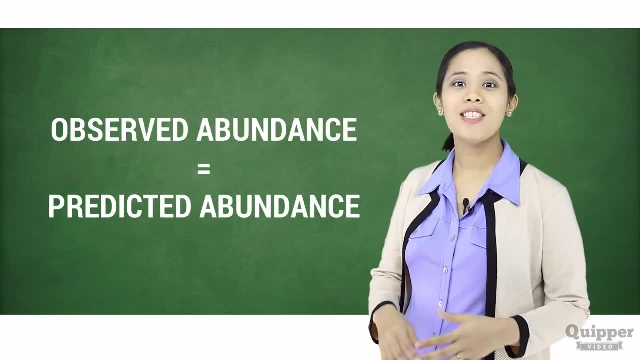 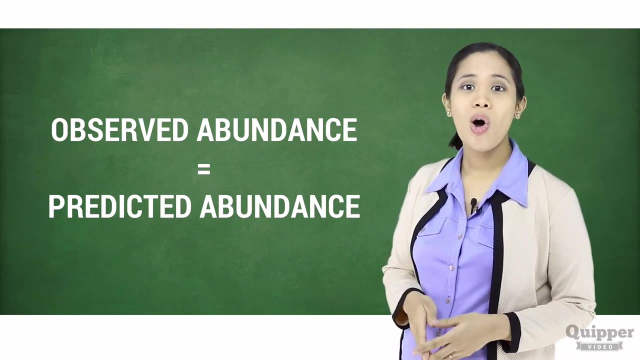 and even less than that would have been lithium and beryllium. Hydrogen and helium were the most abundant elements in the universe. These primordial abundances have been tested. Scientists have measured abundances of primordial material in unprocessed gas in some parts of the universe with no stars.